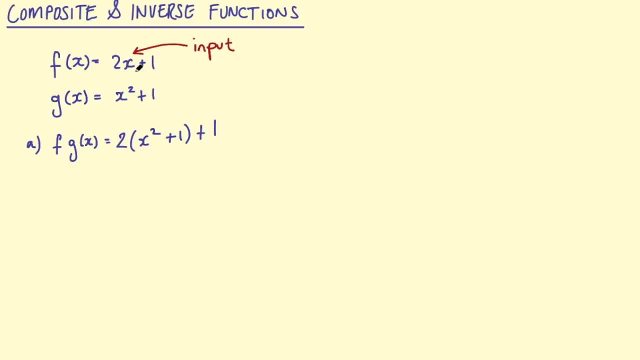 plus 1, and then I have that plus 1 on the end. So I've taken this function and inputted it where the x is in this function here, and then I can just go ahead and solve this. So firstly expand the brackets- this is going to be 2x squared plus 2 plus 1- and then simplify 2x squared plus 3.. 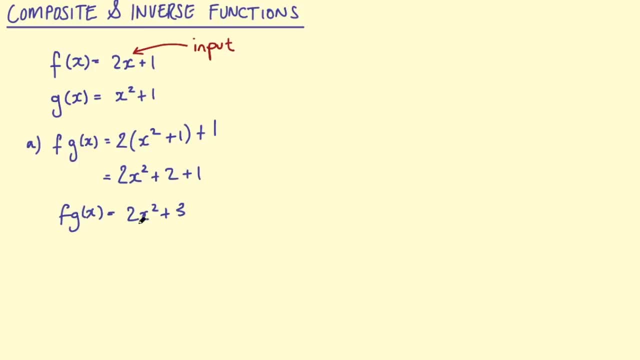 So f of g is going to be 2x squared plus 3.. And we could also do this the other way around. So we could ask for the function of g of f, and you'll notice something about these two functions in a minute. So if we find the function g of f, 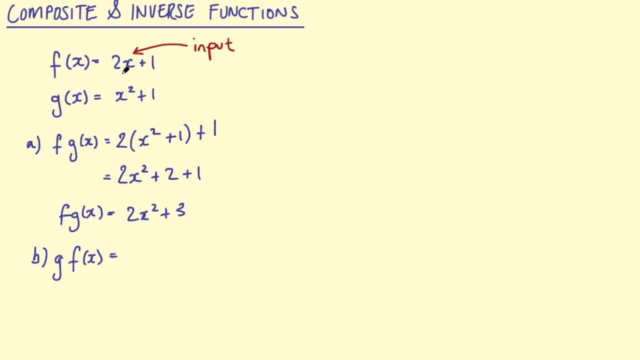 we need to take the function f and input it into the function g. So where this x is, consider this kind of like an empty box or a space where we can put things in- We take this function 2x plus 1 and put it into here. So 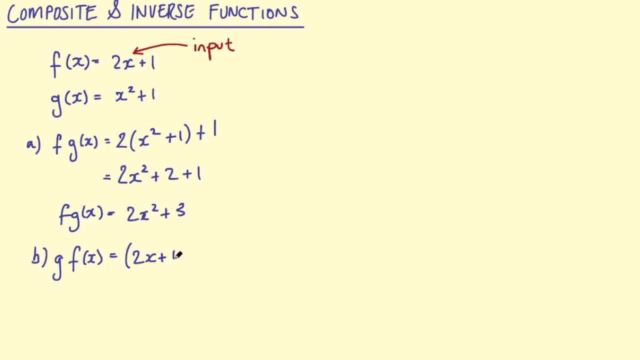 we need to square 2x plus 1 and add 1.. And then we can go ahead and solve this. So expand those brackets out and multiply and we get 2x times 2x, that's 4x squared plus 4x plus 2x squared. 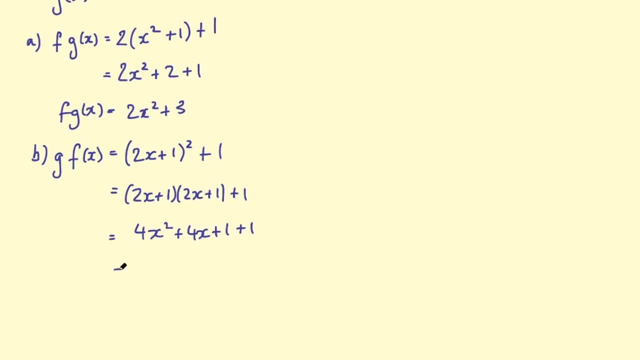 3 x squared squared plus 2x squared x squared plus 1x squared squared x squared plus 1, and plus 1 again, and then simplify So four x squared plus 4x plus 2.. Okay, so now you notice that g of x- uh sorry, g of f is not the same as f of g. 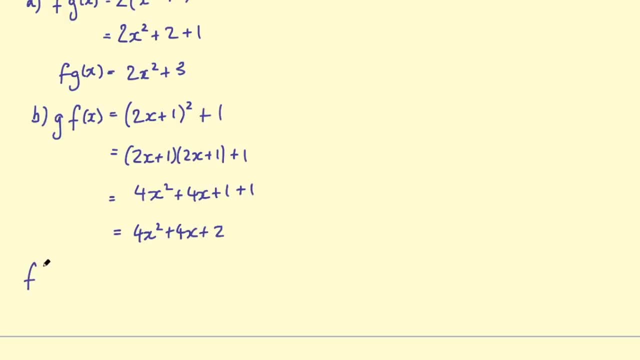 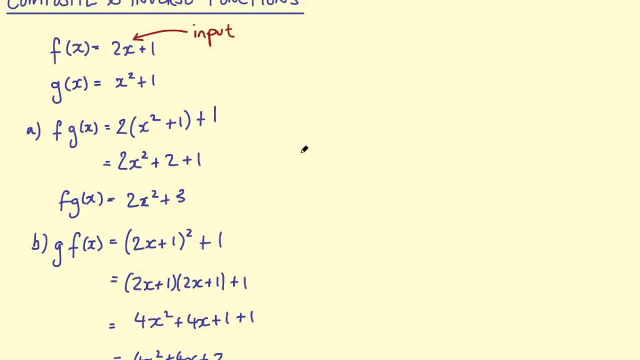 So that's a common element of functions, of composite functions, is that the order matters. so if we take f of g, it's not going to be equal to g of f, and so that's the basics of composite functions. and then questions can get more complicated when you, you know, combine different. 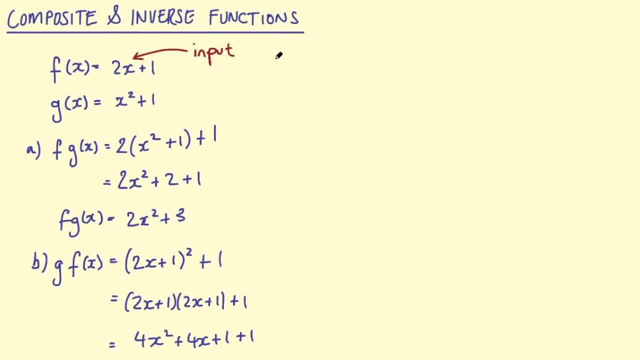 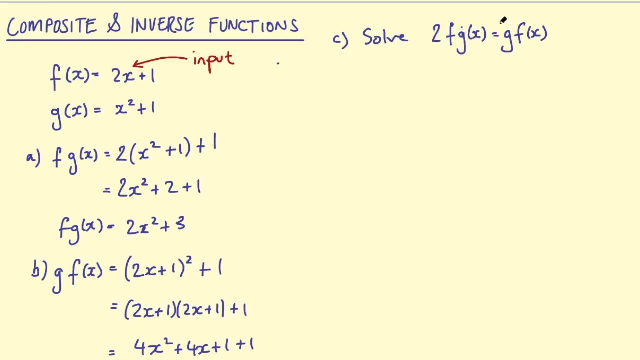 elements of algebra. so we could get a question saying something like: saying something like: solve, solve 2 f of g equals g of f. so here we need to take the solutions to these functions, make them equal and then solve the equation. so i have f of g, that's 2x squared plus 3. 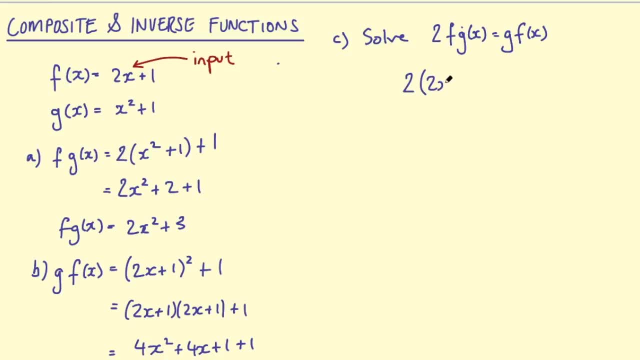 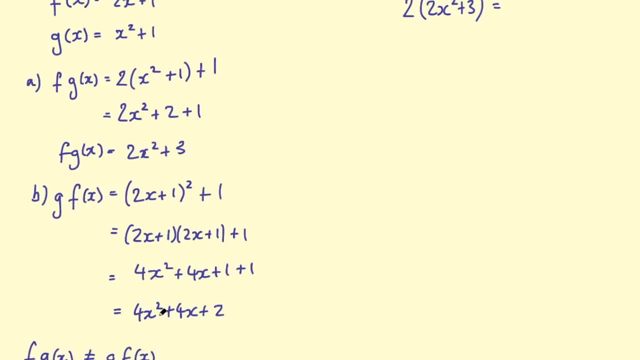 so i need to multiply that by 2, so it's going to be 2 times 2x plus 3. and i also have g of f, which is 4x squared plus 4x plus 2, so that's on the right hand side. 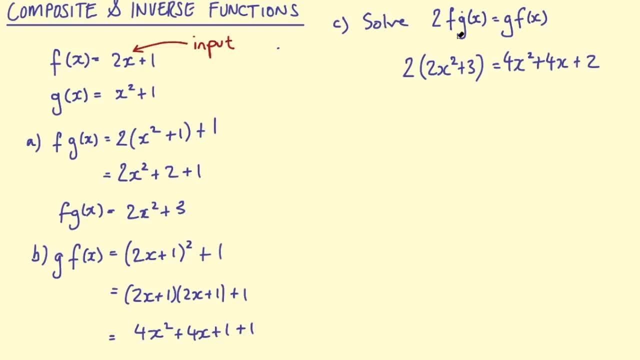 and now i have my equation. i can go ahead and solve this for x. so expand these brackets out first. this is going to be 4x squared plus 6 equals 4x squared plus 4x plus 2, as we have 4x squared on both sides. so if we subtract them, 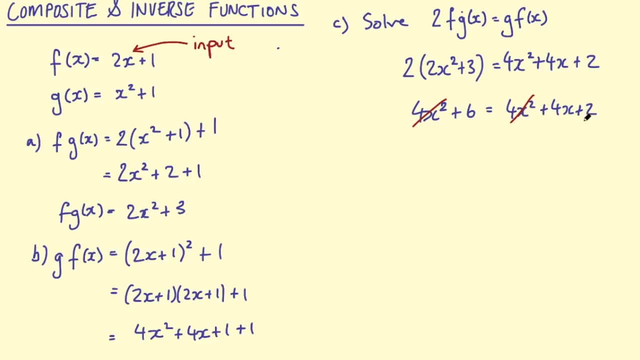 they will cancel out, and then perhaps you could subtract 2 from the left hand side, so we get 4 equal to 4x and then divide by 4. so what we're going to end up with is x equal to 1, and, if you want, 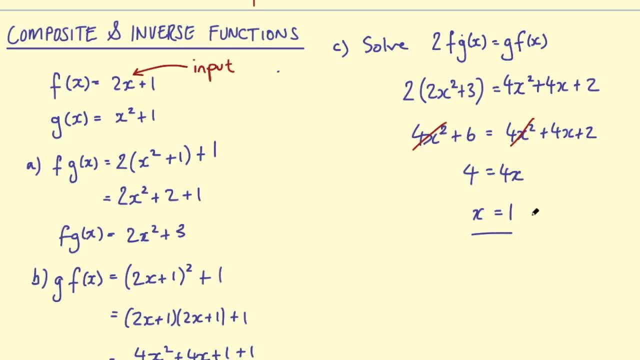 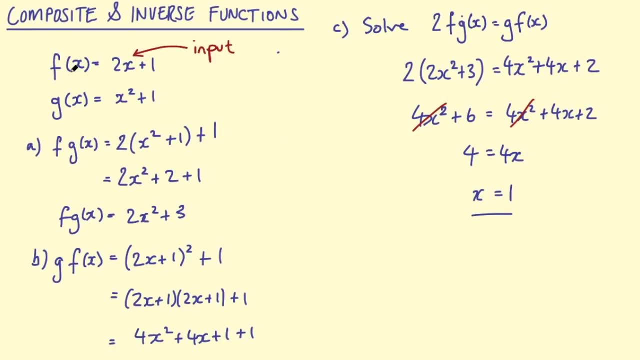 to check that. substitute that into the original equation and you would find that that's the answer. okay, so from this basic element of combining two functions, inputting one function into another function, you can get more complicated looking questions, and this is nothing you probably haven't done. 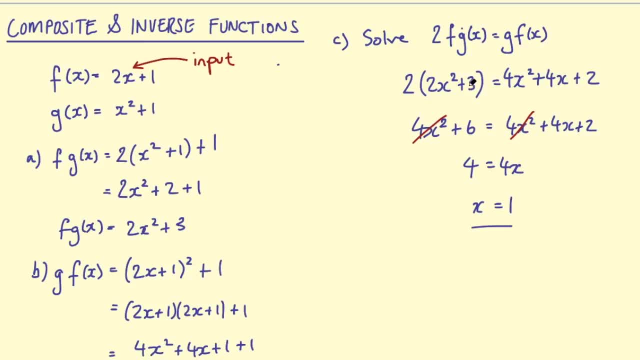 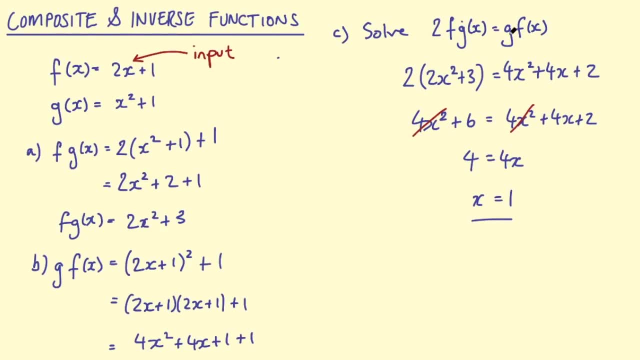 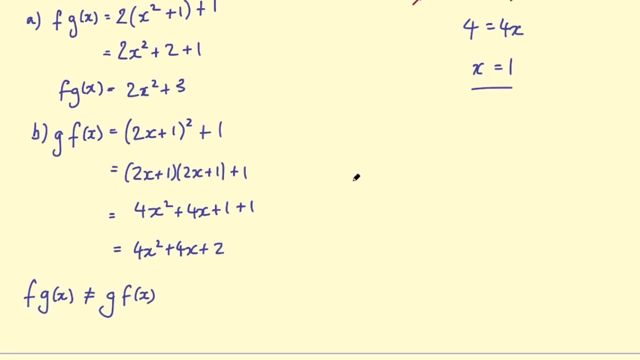 before, which is just solving an equation with one unknown. but i guess the new element is this new notation of using function notation, so it adds just a slight level of difficulty to the question. okay, so now i want to go on and talk about inverse functions, so you can be given a function. 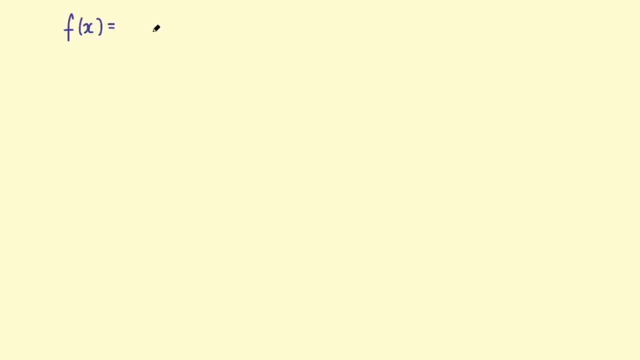 such as f of x or f equals 1 over x, and then you might want to find the inverse of that. so we typically write that as f to the minus 1, which stands for f inverse, and so the first thing we need to do is we say that let f equal y, because the idea of an inverse is that we can take 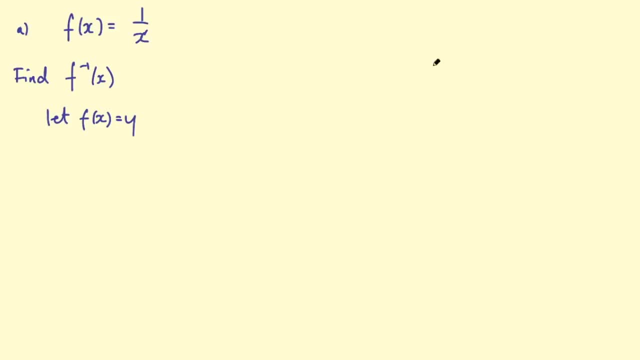 the output and find the input. now, when we're talking about a typical function that gives us the output, given any input, and what the inverse function does is gives us the input given any output. so we first thing we do is we let f of x equal y, in other words the output, so we can say y equals 1 on x and rearrange. 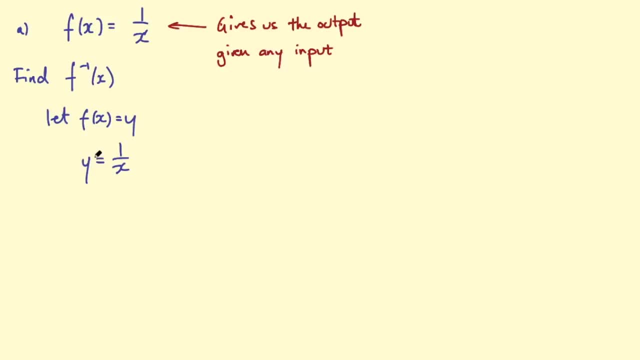 to get x by itself. so in this case we'll multiply this side by x, so xy equals 1, and then divide by y, so x equals 1 on y. and now what this equation is doing is saying: if we input y, we will get x. in other words, if we 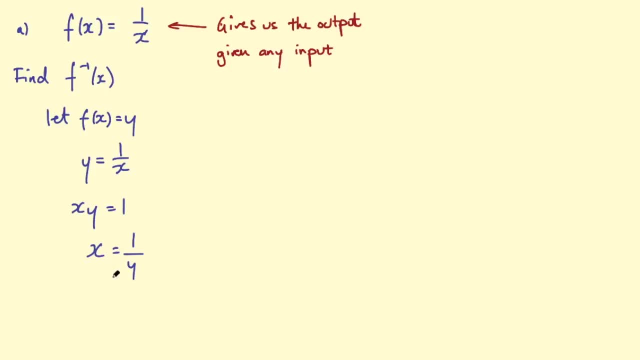 input. what we originally called the output, we will get the input. so that's the idea of an inverse function. and so now we change the letters so the, the output, becomes the input. in other words, the output becomes x, so we call this f- inverse f to the minus 1 and the y becomes the input. so this is going to be. 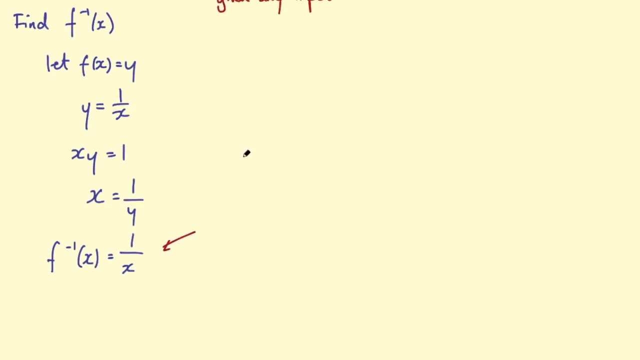 1 on x. so this gives us the. so this gives us the input of the original function, given any output. so you can see it's just the opposite or the inverse of the original function. I hope that makes sense. so let's just do one other example. 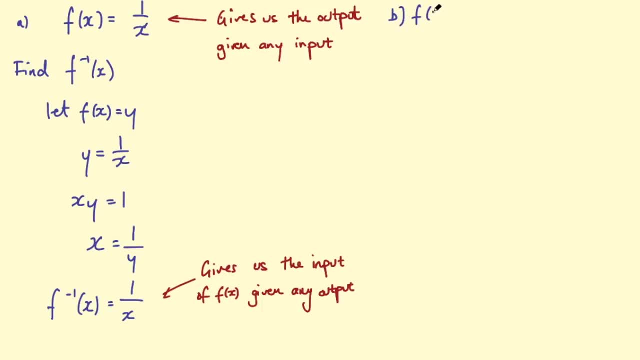 of this. so you you might be given a function like 2x minus 4 and you're asked to find the inverse. so remember, the first step is to let f equal y and then say y equals 2x minus 4 and then rearrange for x, so add 4 to the left hand side, so it's going to be y plus. 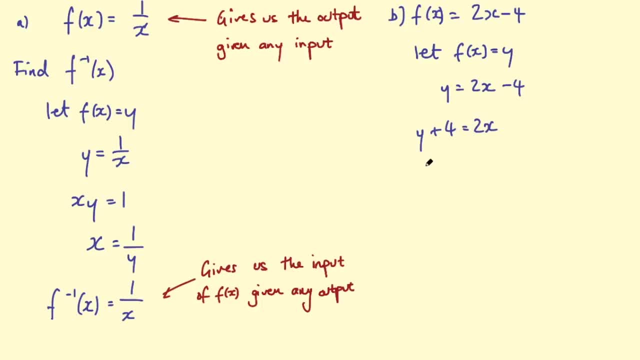 4 equals 2x, and then divide by 2, so y plus 4 divided by 2 equals x, and so x equals y plus 4 divided by 2. and now remember that y or that output becomes the input, and we call this the inverse function. so we can: 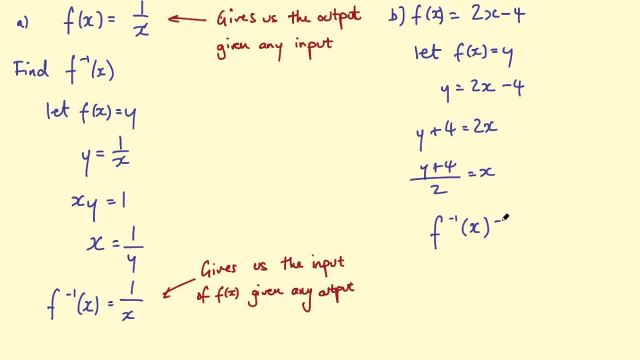 say, f inverse equals x plus 4 divided by 2, and that's pretty much the method you can use in in all cases when you're asked for an inverse function. so as long as you practice that method, you're going to be able to find the inverse function. 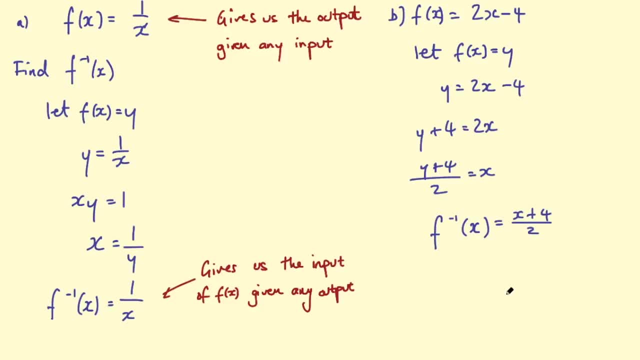 so if you've used that method enough and you can understand it and remember how to do it, then you'll be fine with questions on inverse functions. and then they can just get slightly more difficult, so you can get questions such as this one where you're given f which 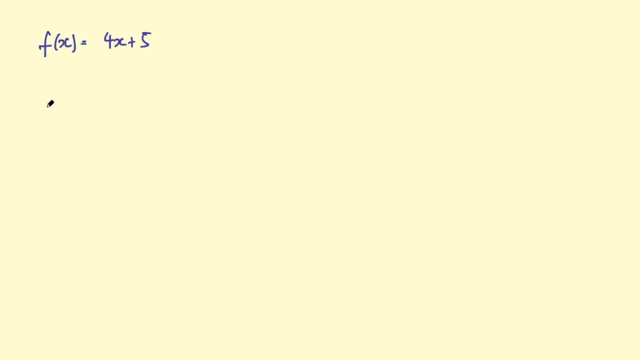 is 4x plus 5, and they asked you to prove that f of f inverse equals x. so this is a key to doing this in the first phase. OK, well, this Donna was asking you to first find the inverse function and then input that into XYZ. 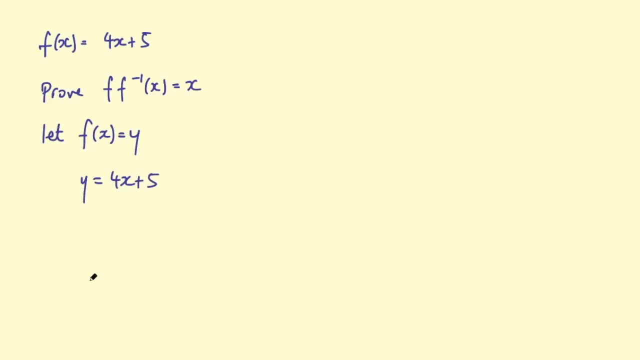 so the first thing we have to do is to find the inverse function and remember that that means letting f equals x, and so we can say y equals 4x plus 5 and then rearrange to get x by itself. So this is going to be y minus 5 on 4 equals x. 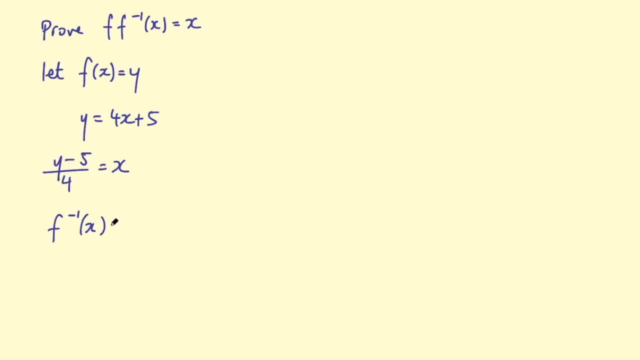 So subtract that 5 divided by 4 and then array for x equals 4 divided by 4 divided by 4, and then therefore f inverse equals x minus 5 divided by 4, and now we want f of f inverse. So we take: 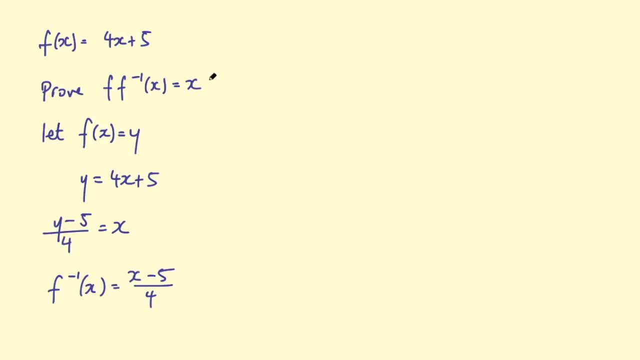 this function and input that into the original function. So f of f inverse, and we can change that input to be x minus 5 on 4, and this is going to be 4 times x minus 5 on 4 plus 5. and now we 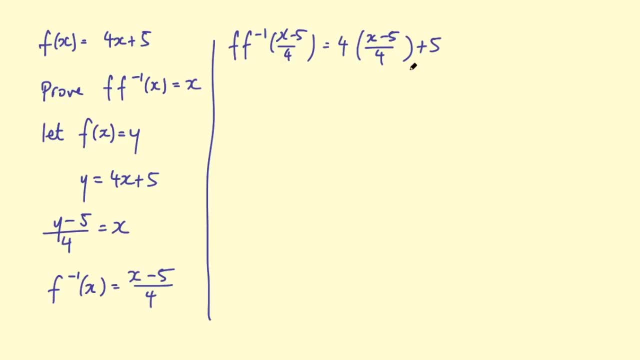 just need to simplify this right hand side. So 4 multiplied by this fraction, well the 4, 4 divided by 4 is just 1, so we can cancel those 4s out and on the next line we are just left with x minus 5. 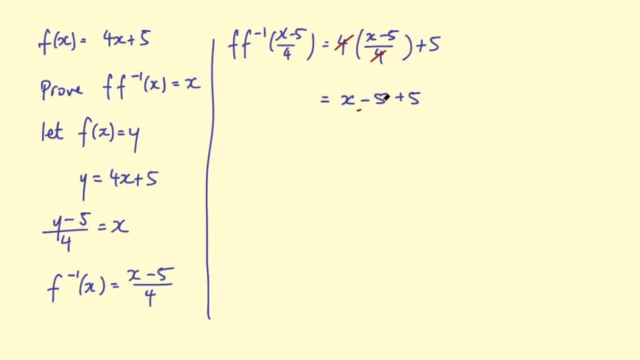 plus 5 or minus 5 plus 5.. That's 0, so we're just left with x, and so therefore we can say: f of f inverse equals x. So we've proven what they've asked us to prove. and lastly, you can get questions such as this one: 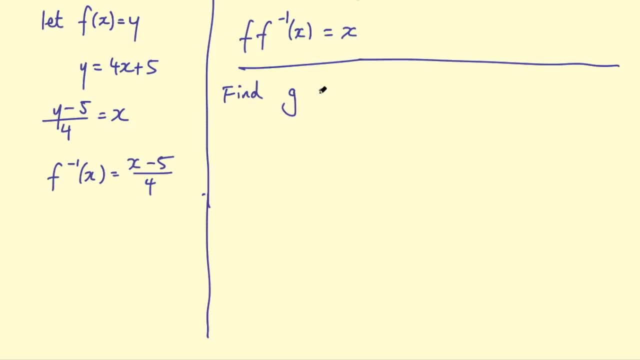 So it might say: find g, given g equals mx plus c and the function f equals 2x plus 3 and f of g equals 6x plus 7.. This is saying that the function g must be a straight line. Remember, this is the general equation. 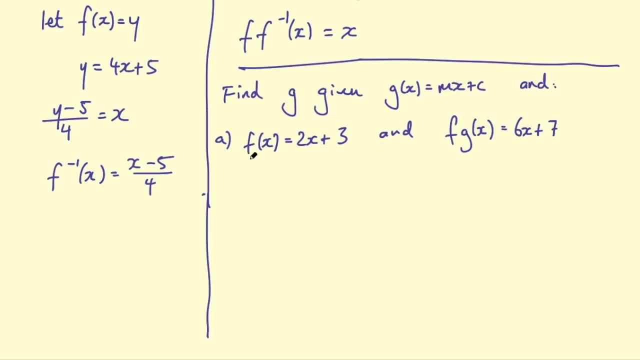 of a straight line mx plus c and were given a new function f and we're told: and when we input the function g into f we get 6x plus 7.. to find the function g, we can input this general equation into f, so we can say that f of g. 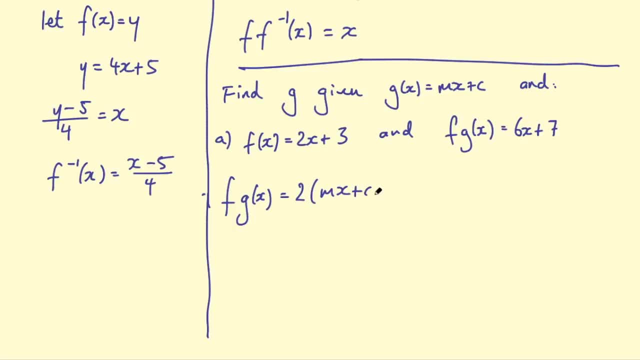 will be 2 times mx plus c plus 3.. So I've taken this here and inputted it into f of x, where the x is right. so I've got 2 times mx plus c plus 3, and then start to simplify this. so this is going to be 2mx plus 2c plus 3. 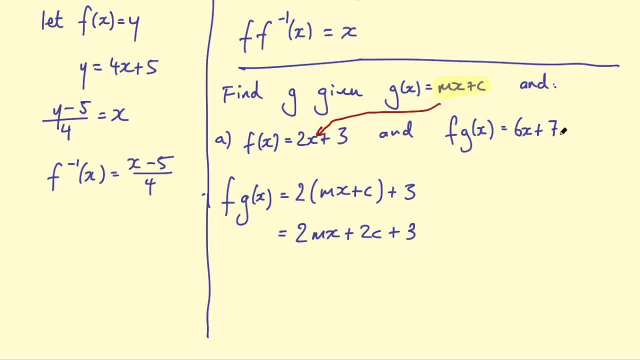 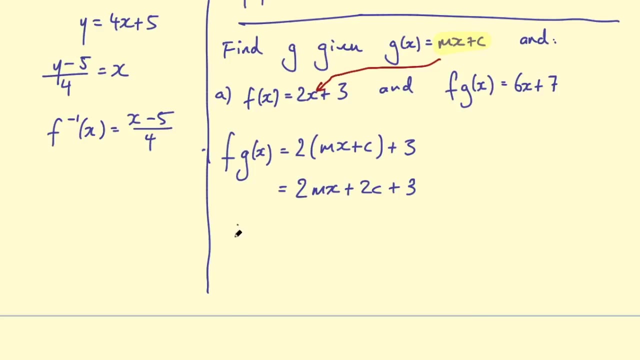 and we're also told that f of g equals 6x plus 7.. So I have an expression here for f of g which I can make equivalent to this expression up here Now. in this expression, 2mx will be equivalent to 6x. so therefore I can say that 2m equals 6. 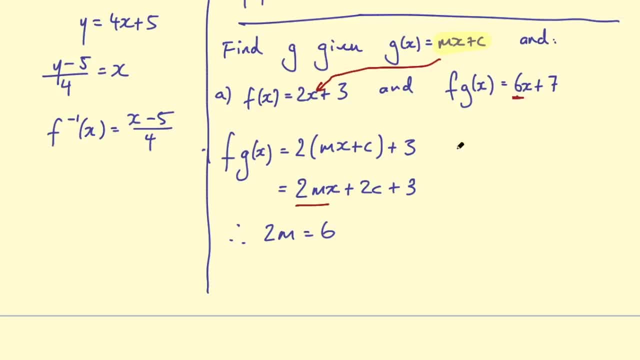 so this coefficient of x must equal this coefficient of x, because these are the same functions f of g. So that allows me to say that m equals 3, also 2c plus 3 must equal 7.. So that allows me to solve for c. so 2c equals 4, so c must equal 2, and so I have m, I have c, so there's.